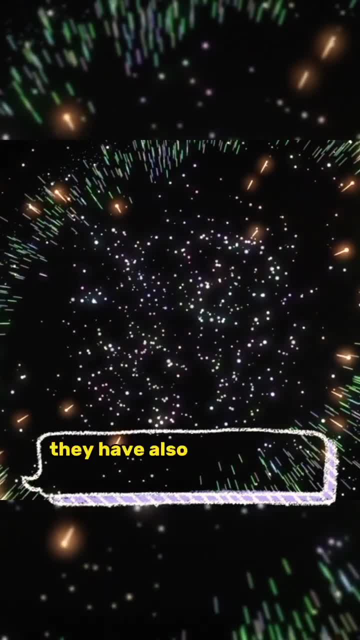 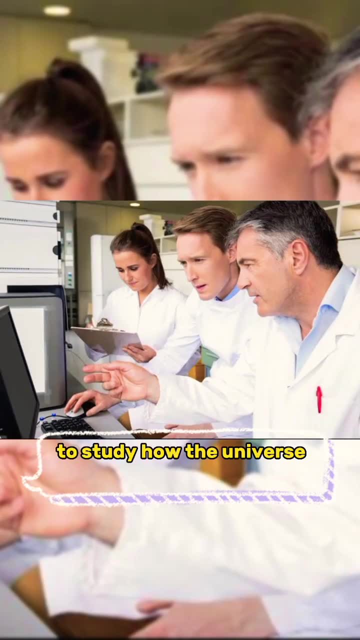 which is leftover radiation from the Big Bang. They've also looked at the distribution of galaxies and stars in the universe and used computer simulations to study how the universe has evolved over time. So there you have it: the Big Bang Theory explains the origin of the universe. 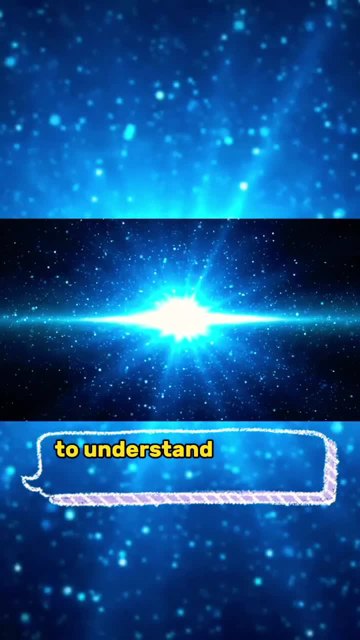 And scientists have been studying it for years to understand how our universe came to be. 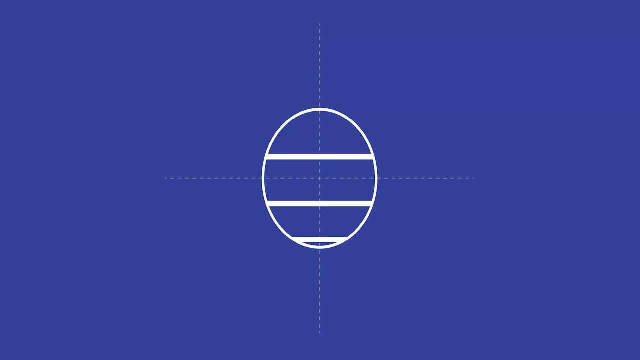 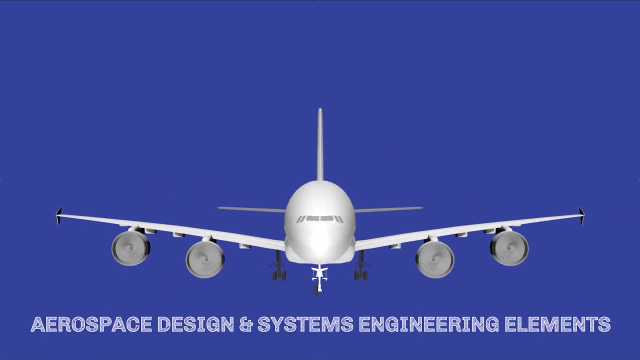 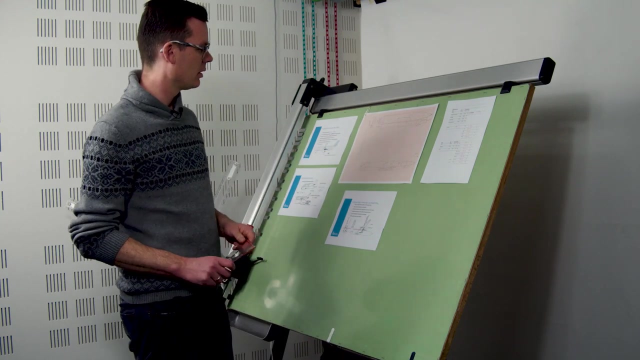 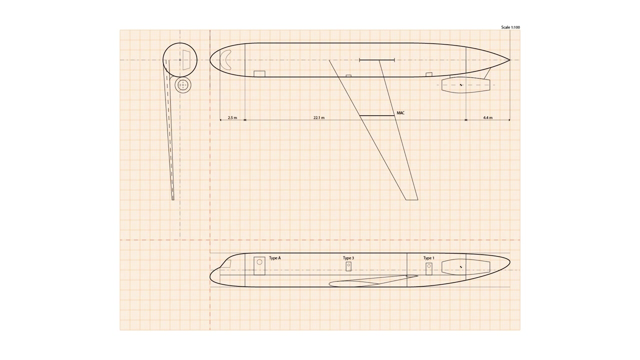 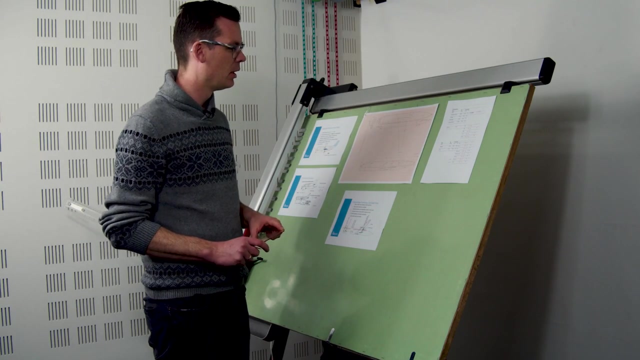 In this video we are going to position the landing gear. We are looking at this, this starting point, where we have the airplane with the the wing already installed, so that the CG analysis has already been done and the the wing has already been positioned in this phase. So there is a couple of deviations with 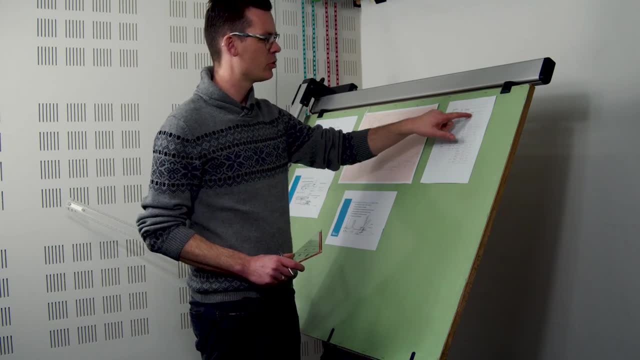 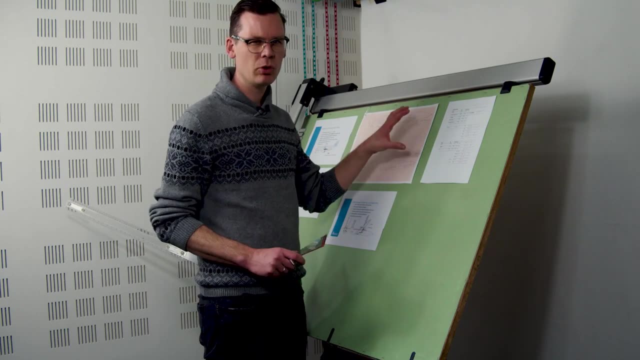 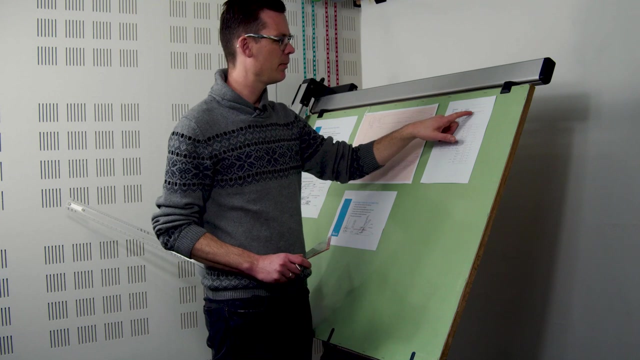 respect to the exam of 2019.. In that exam, we had assumed a position for the for the engine. In this exercise, you saw, I actually drew in the engine, which led to a slightly different position. So we start with an engine which is a little bit more off than on the exam. It's about 77% of the fuel. 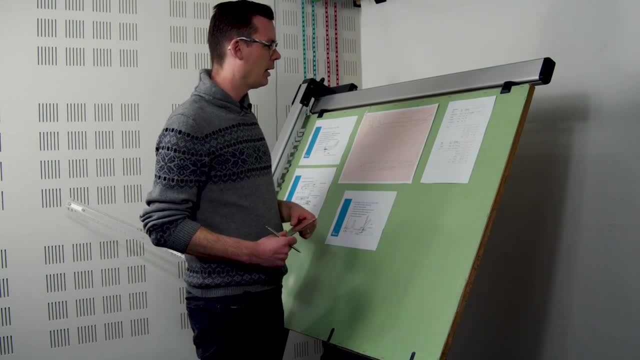 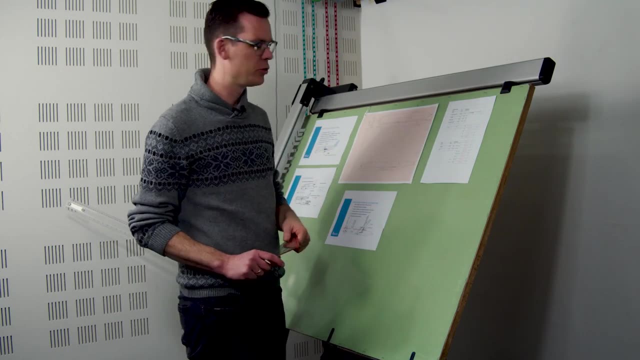 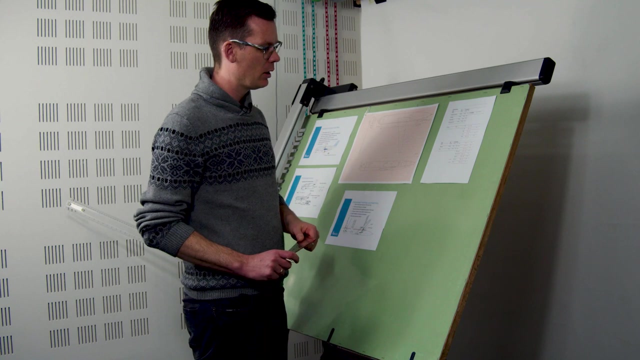 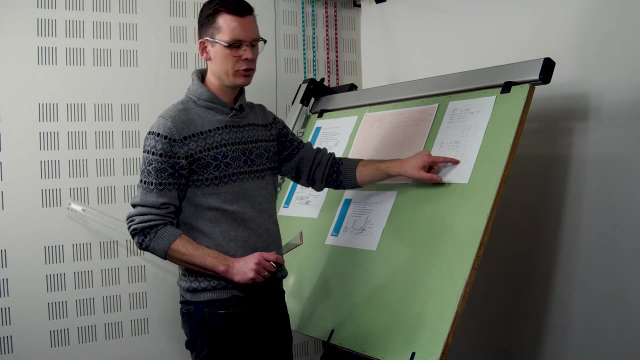 that's a large length and at least that's where the CG actually resides, and that also gives a little bit different results downstream and also results in a slightly more half located wing position. We put the all the the calculations were performed, The sheet has been filled out and from this sheet I am starting with.